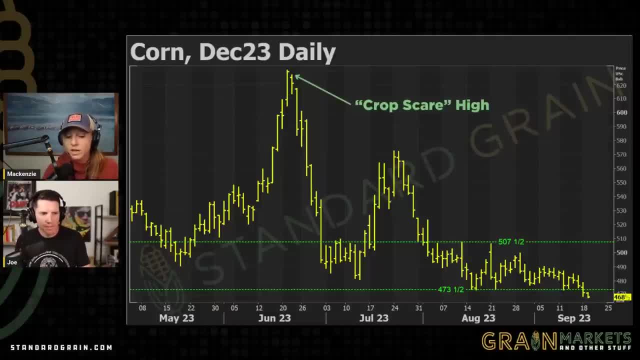 lows. yesterday, after holding the 473 area on multiple occasions, The December 2023 contract finally fell below key support. Seasonal pressure paired with a lack of export demand and river issues pressured the market. USDA projections indicate the most bearish US supply and demand. 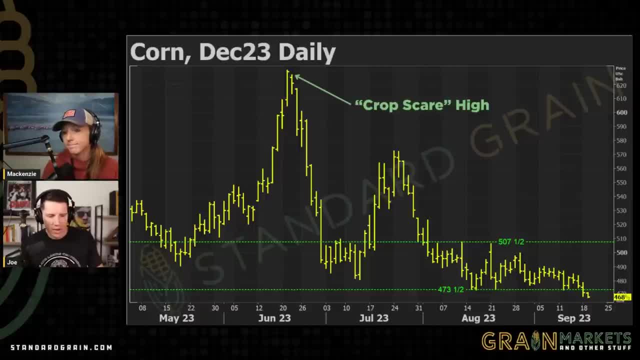 situation since 2018.. Okay, When McKenzie said the most bearish US supply and demand situation since 2018, we're using stocks to use ratio as our metric and that is the best metric for gauging supply and demand. In 2018, we were a 15 and a. 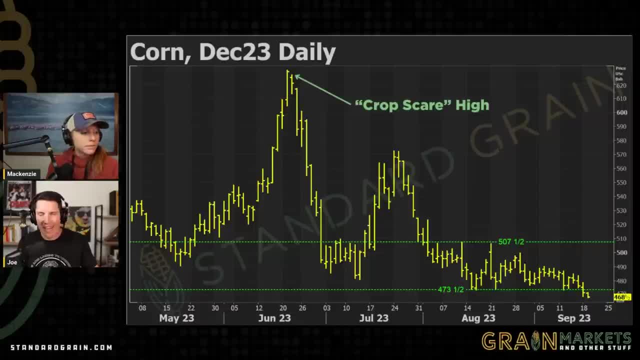 half percent stocks to use ratio domestically. The projection right now is 15.4.. And you guys remember 2018 corn prices were not at 464.70.. Your lows were in like the low $3 neighborhood, So we're down to 468.. 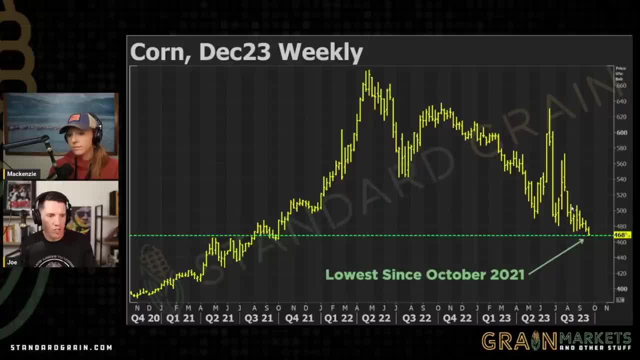 We're down to 464.. We're down to 466.. So we're down to 468.. So we're down to 464.. So we're down to 469.. So we're down to 468.. Now, as we tape here this morning, which is fresh low for this move. 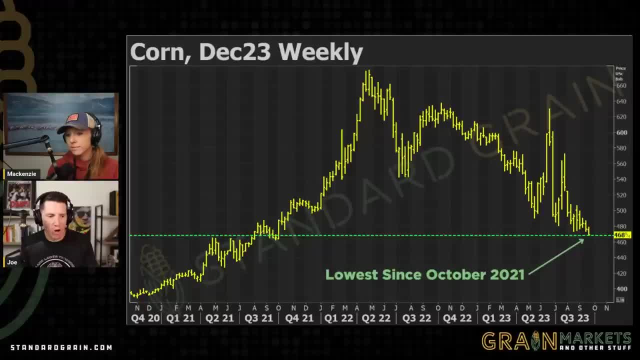 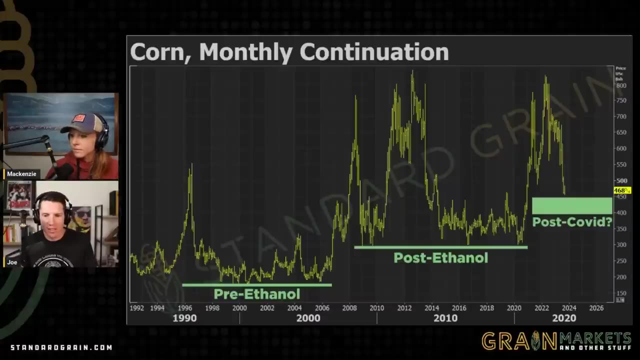 If you peel back the December chart, this is the lowest trade for this December 2023 contract since October of 2021. So you got to go back a long ways. The million dollar, or perhaps billion dollar, question for me in this environment is: what is a cheap corn price in 2023?? And I threw this chart. 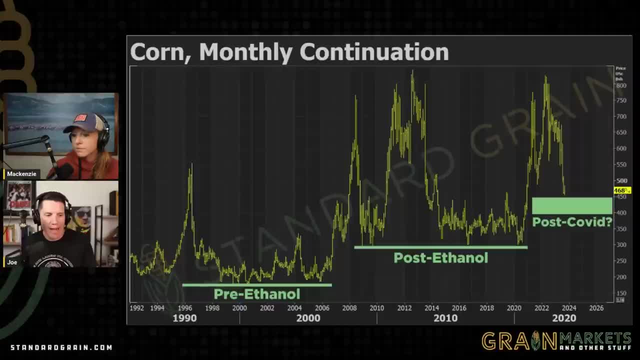 together. I think this is a good way to to maybe lay Yep decades. So. prior to the US ethanol boom, the low end of the corn market was like $2 down to maybe $2.75, somewhere in that neighborhood. You would very frequently bottom in that neighborhood. 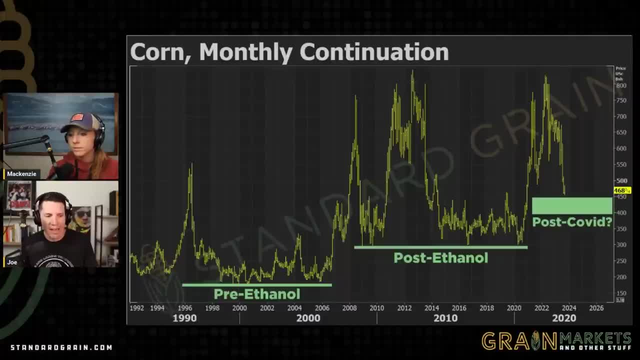 but never below that neighborhood. Then you had the ethanol boom 2006, 2007.. After that time frame you almost never saw corn below $3. You had kind of a new low end of prices. When things got really bearish, $3 was like the low end of your trade in the corn market. Now we are in what? 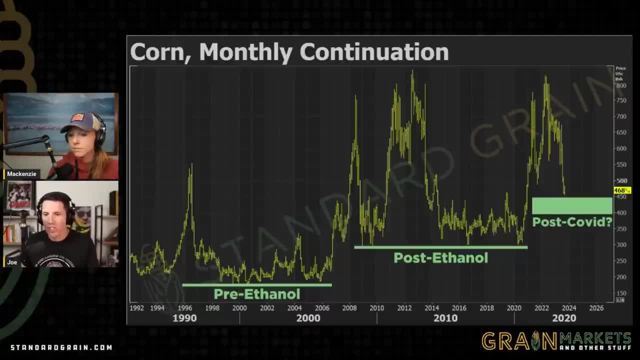 I would call a post-ethanol, post-COVID, post-inflation environment And COVID. the virus itself doesn't matter, but the money printing, the low interest rates, the inflation absolutely does matter, And all of those things were a result of COVID, I guess. So the way that everything on. 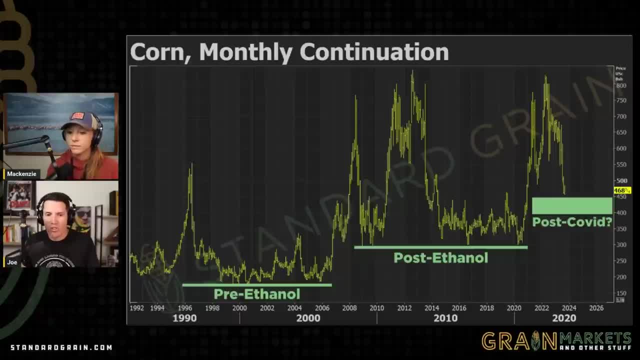 the planet is priced. everything's increased by 20,, 30,, 40, 50% over the last three years. So what is the new low end of corn prices in this post-COVID environment? That's the billion dollar question. And I think when you step back from the daily headlines about export sales and 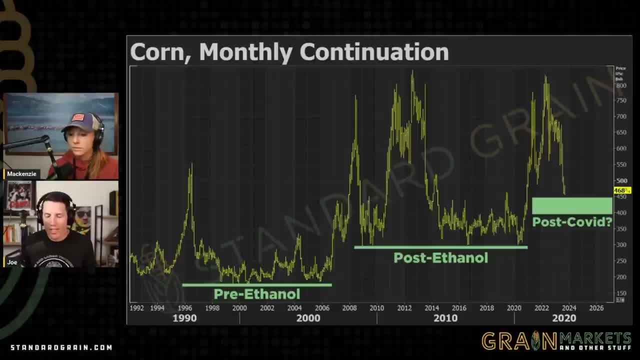 USDA reports, and how big is the crop? this is the question that we will seek to find the answer to And, given the fundamental setup, we may very well find the answer this year. unfortunately, I hope it's somewhere in the $4.50 neighborhood and not $4.00.. And who's to say that it's? 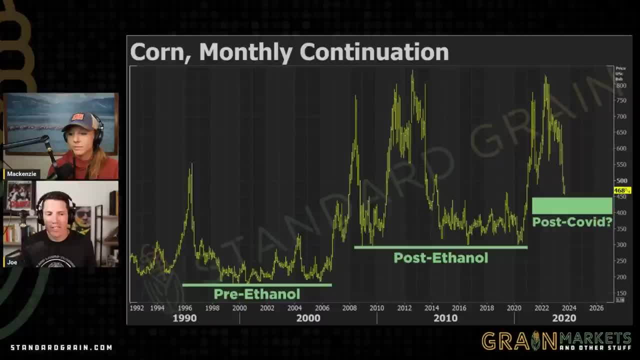 not still $3.00? I don't know, but this is one of the biggest questions out there as it relates to corn prices. at least for me right now. I just think that, given the supply and demand situation, it's pretty bearish. but what's a cheap corn price in 2023? I don't know, but we may find out. 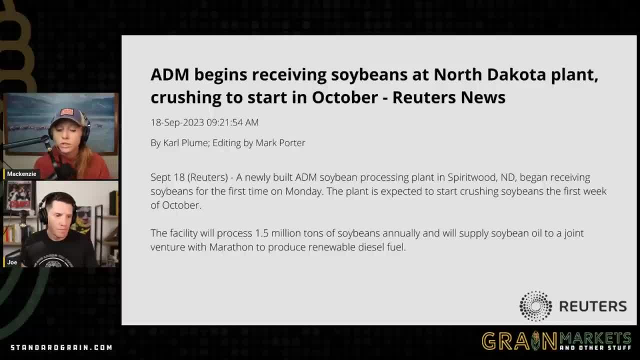 A new ADM plant will soon start crushing soybeans. The plant, which is located in Spiritwood, North Dakota, began receiving soybeans for the first time on Monday and will begin crushing by the first week of October. The plant will provide soybean oil to Marathon as part of a joint venture to produce renewable diesel fuel. 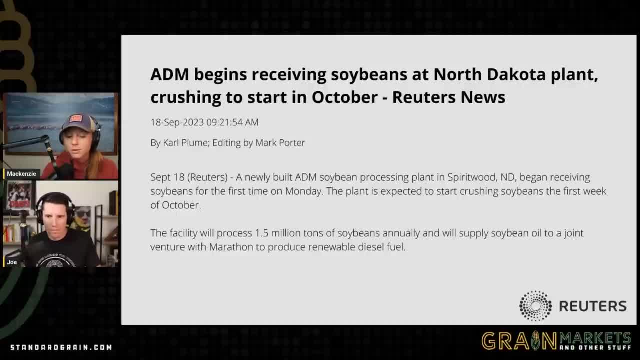 The facility is expected to process 55 million bushels of soybeans annually. ADM is working to bring some of the affected areas back to safe operations after the explosion at the Decatur plant last week. Yeah, I haven't heard much about the Decatur plant. I was checking ADM's website. 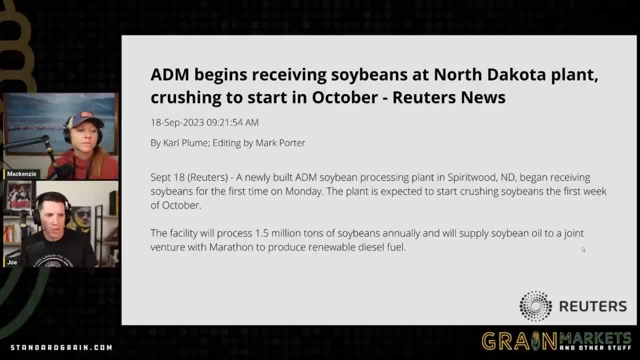 for news releases and I don't think there's been an update. Spiritwood, North Dakota, is along I-94 between Bismarck and Marathon. There's been a lot of talk about it, but I don't think there's been an. update. Spiritwood, North Dakota is along I-94 between Bismarck and Marathon. There's been a lot of talk about it but I don't think there's been an update. Spiritwood, North Dakota is along I-94 between 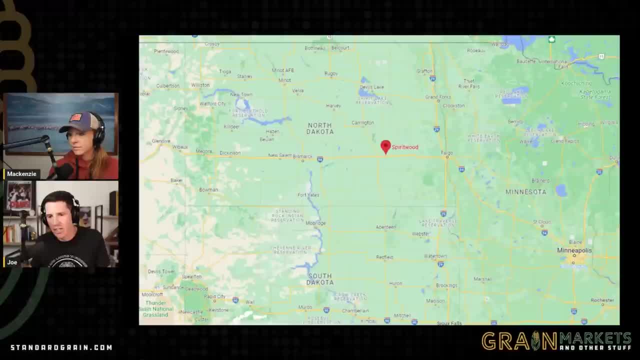 Bismarck and Marathon. There's been an update. Spiritwood North Dakota is along I-94 between Bismarck and Marathon. There's been an update: Spiritwood North Dakota is along I-94 between Fargo- I guess a little bit closer to Fargo. This will be really good if you guys are in that area. 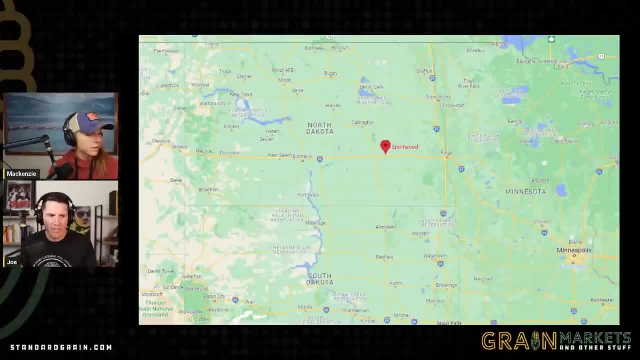 There's been an update. Spiritwood North Dakota is along I-94 between Bismarck and Marathon. There's been an update. Spiritwood North Dakota is along I-94 between. should be good for basis, just general demand to have some more competition If you guys are in. 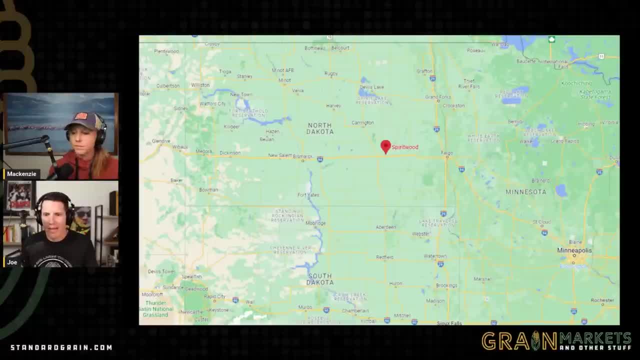 that neighborhood and you have any sort of update as it relates to basis, maybe this year versus historical, let me know. I don't know if it's going to be really great, given some of the issues on the river and things along those lines, some of the lack of demand problems, But this is overall. 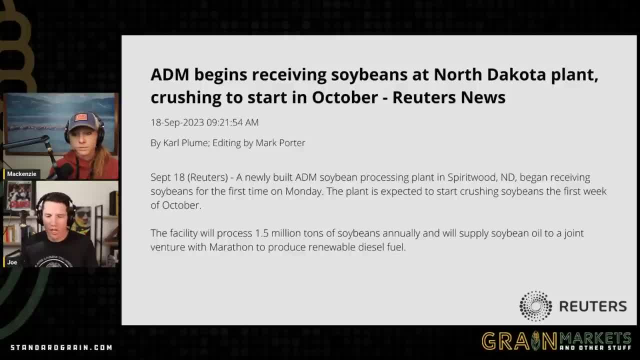 a big positive- and these crush expansion stories- we talked about this a little bit yesterday following the crush report. You're going to continue to see headlines along these lines- new crush plant opens or new capacity opens, things along those lines here over the coming. 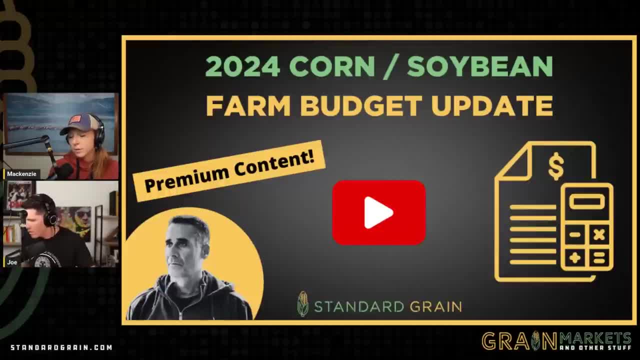 months. I guess If you guys are not already subscribed to our premium content, you sure need to do so. Joe, can you tell me about the video you put together yesterday? Chris Barron from AgView Solutions, who is a regular contributor, was on with me yesterday. 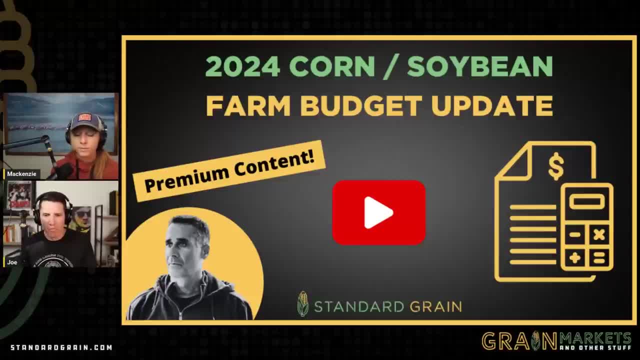 We talked about 2024.. Corn and soybean farm budgets. If you guys are not budgeting, this is absolutely the year to start, because 2024 could be a very, very tight margin year. We've been privy to some really good margin. 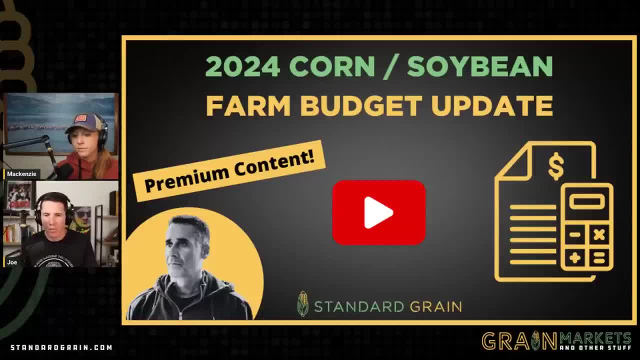 years where corn prices, soybean prices, were above the cost of production for two, three years straight. And now we're in an environment- potentially we could be entering an environment- where we straddle the cost of production. Maybe you spend time below it. maybe you spend time. above it. Chris Barron from AgView Solutions, who is a regular contributor, was on with me yesterday. Chris Barron from AgView Solutions, who is a regular contributor, was on with me yesterday. Maybe you spend time below it. maybe you spend time below it. maybe you spend time above it. 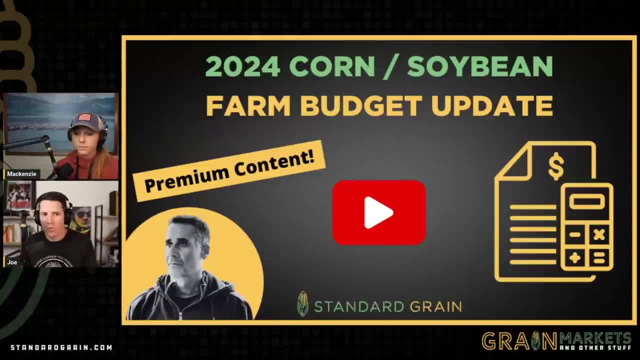 Chris Barron from AgView Solutions, who is a regular contributor, was on with me yesterday. We're below the cost of production for a lot of you guys For 2024, there may still be some black ink available on the budgets. Chris ran through an aggregate of his customer base as it relates. 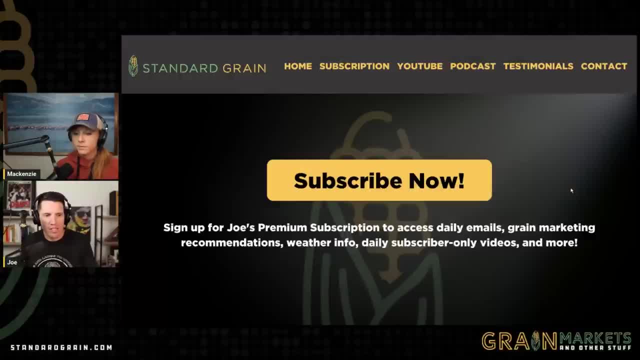 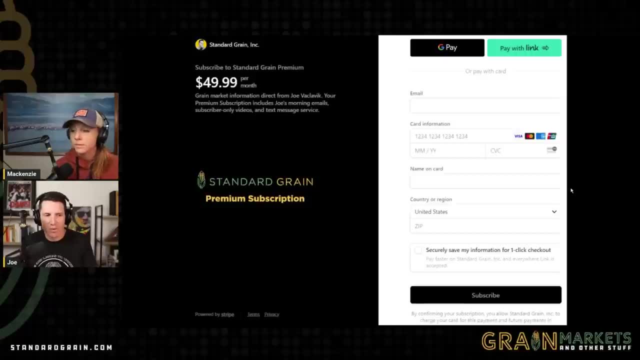 to production costs. We ran some best practices. If you guys want to see this video and all the other premium stuff, go to standardgraincom. You can sign up this morning. It takes one minute to sign up. You can do it on your phone or on your computer. It's a $50 per month subscription. 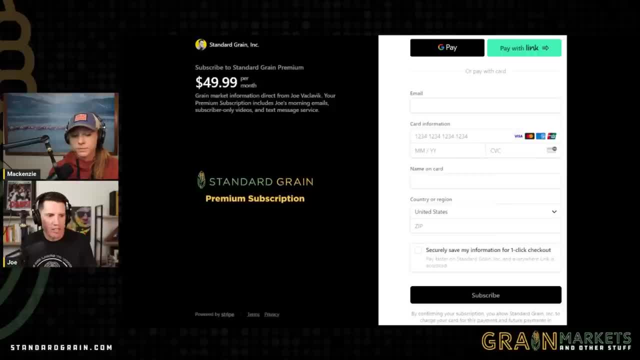 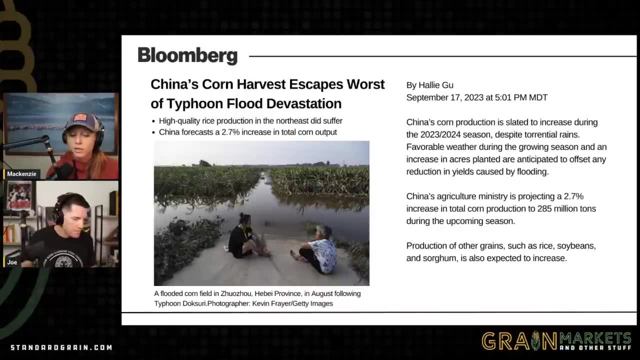 Cancel it any time. No other fee, no other obligation. Nobody will try to sell you anything else. Check that deal out this morning, guys. China's northeastern region is expecting an increase in corn production, despite heavy rains, Favorable weather and an uptick in acres planted. 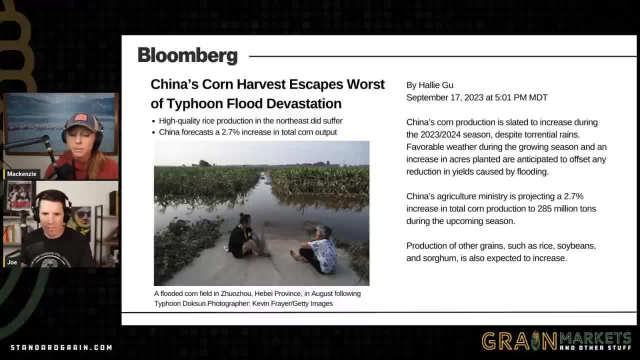 will likely offset any damage to yields caused by the torrential rains. Some areas that experience flooding are expecting to have corn yields cut by as much as 10%, according to China's ag ministry, Total corn production during the upcoming season, which officially begins on October 1st. 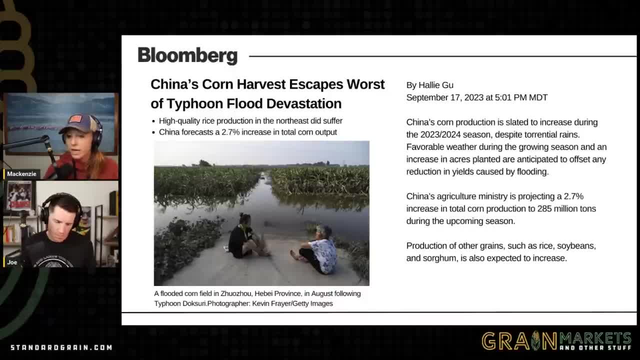 is projected to rise 2.7% to 285 million tons. China- the Chinese government- is higher than USDA. USDA is at 277.. China is at 285.. In either case, it's a huge crop And we've 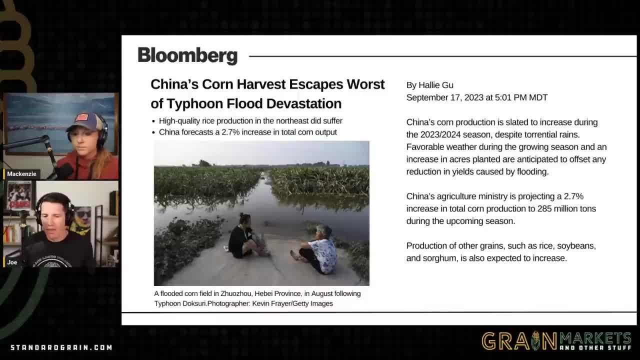 talked about this story in the past, thinking maybe if the damage is widespread enough, that there's enough. maybe that means China has to come buy US corn or they just need to import more in general, And that just doesn't appear to be the case. USDA is at 277, and USDA's. 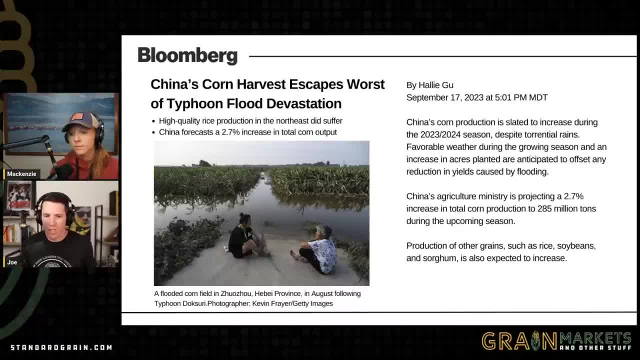 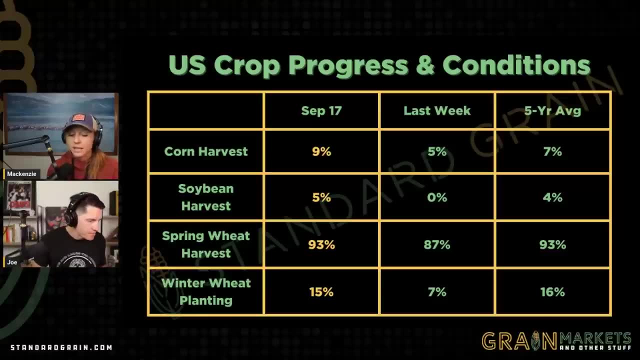 projection of the record crop previously was 277.2 from last year, So they're talking a near-record crop, just fractionally below last year. So yeah, there was some damage, but not enough to really put a dent in this thing. the way that it looks, US corn harvest is slightly ahead of schedule. 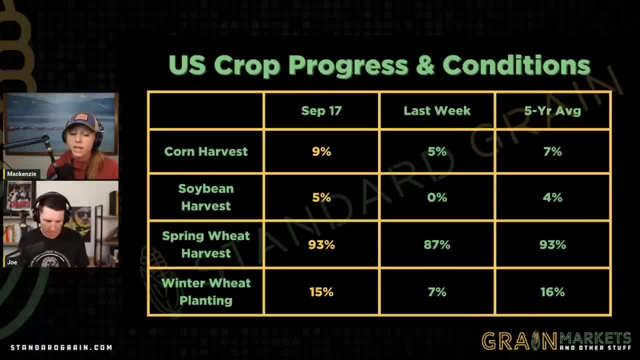 The crop was 9% harvested nationally through Sunday, compared to 5% the prior week and 7% on average. States that have harvested 20% of the crop or more include Texas, Kansas, Tennessee, North Carolina and Kentucky. Corn conditions dropped to 51%: good to excellent. 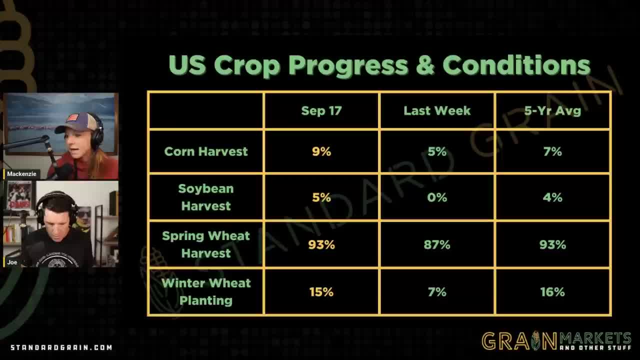 nationally from 52% the prior week and 59% on average. Go ahead and do soybeans too. Okay, so US soybean harvest has kicked off. The crop was 5% harvested nationally through Sunday, compared to 4% on average. States that have harvested 20% of the crop or more include Texas. Kansas, Tennessee, North Carolina and Kentucky. Corn conditions dropped to 51%- good to excellent- nationally, from 52% the prior week and 59% on average. Go ahead and do soybeans too. Okay. so US corn harvest has kicked off. The crop was 9% harvested nationally through Sunday. compared to 5% the prior week and 59% on average. Go ahead and do soybeans too Okay. so US corn harvest has kicked off. The crop was 9% harvested nationally through Sunday, compared to 4% the prior week and 59% on average. Go ahead and do soybeans too, Okay. 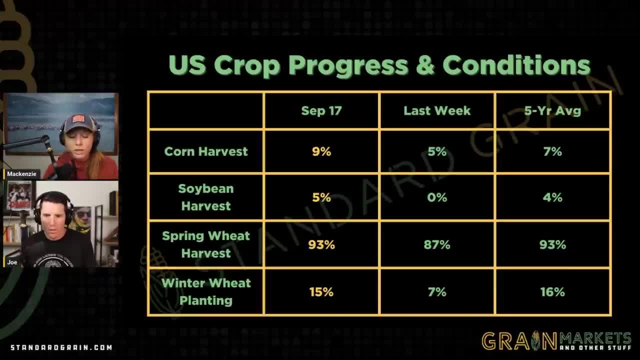 that have harvested 10% of the crop or more include Louisiana, Mississippi, Arkansas and Tennessee. Soybean conditions were unchanged nationally at 52% good to excellent. So yesterday you had kind of a nasty sell-off in the soybean market. Corn posted some fresh lows. 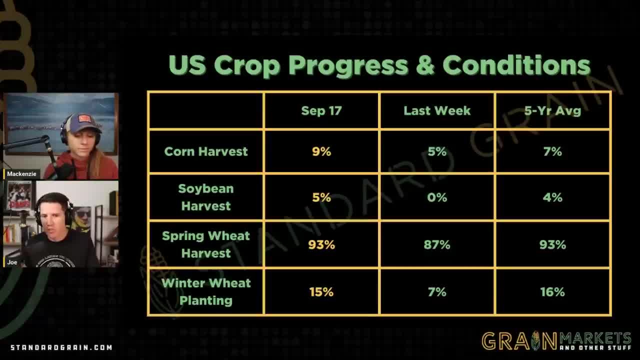 You could call it harvest pressure. It could be some early harvest pressure or seasonal pressure. The market is not supposed to act good on average over time during August, September and then, in the corn market in particular, your harvest, low on average over time, will occur on October 1st. 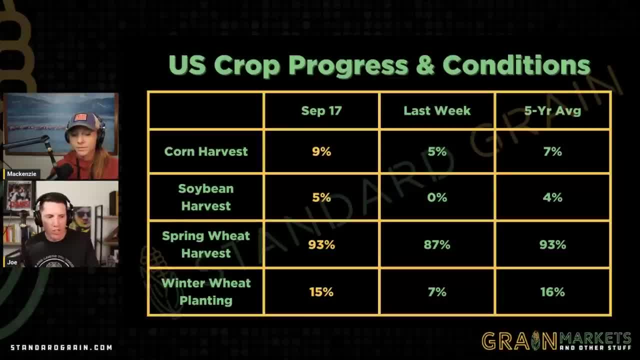 but that's different every year. Seasonals certainly don't always work, but things are moving along. where we've seen the most progress, of course, is in the South, and there is activity going on this week. so things pushing forward. What about winter wheat? So wheat planting is. 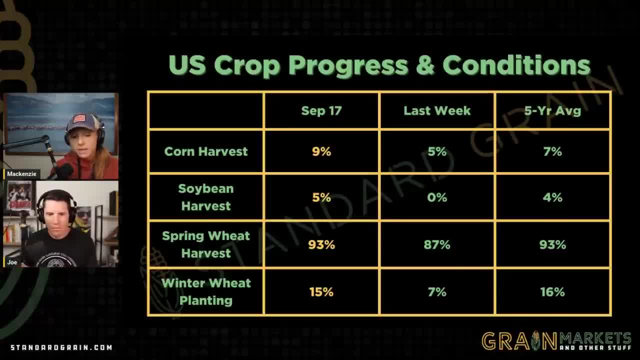 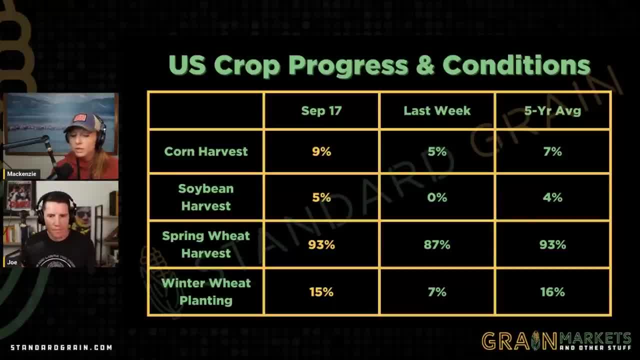 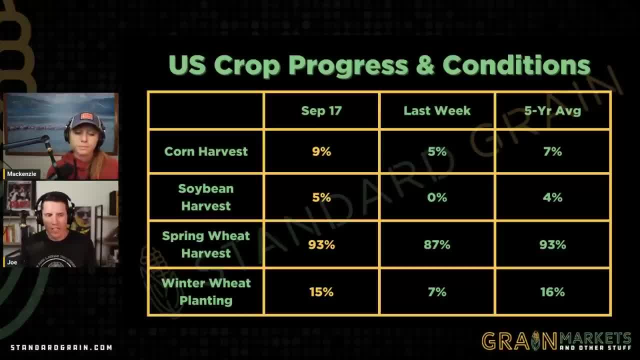 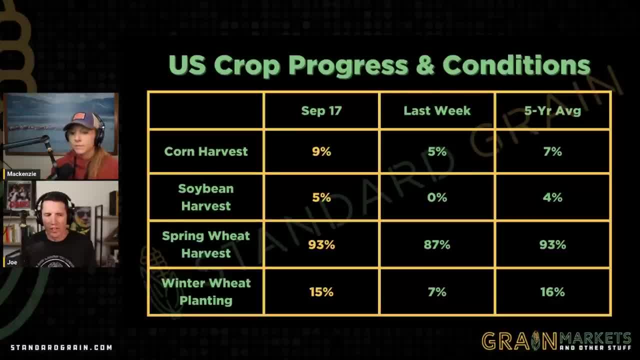 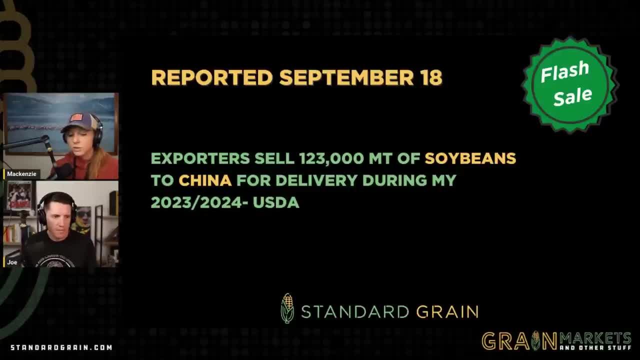 newsletter on Friday. We had an export sales chart in the newsletter on Friday. The Book of US wheat export sales is like the worst in more than 20 years. We could really use some wheat demand. That would be helpful. USDA reported a flash sale of US soybeans on Monday. 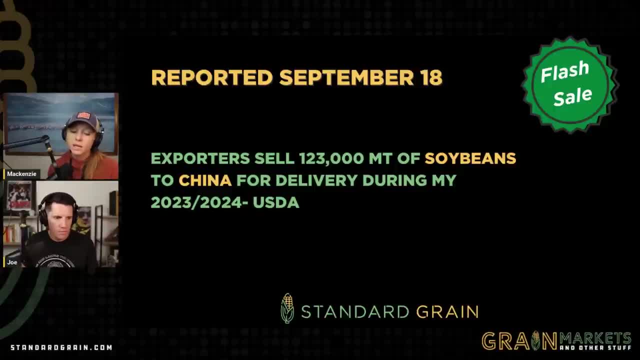 US exporters sold 123,000 metric tons of soybeans to China for delivery during the current marketing year. The sale is regarded as routine business. Yeah, that's the buyer you want to see, but not necessarily the amount. We would like to see some bigger business reported to. 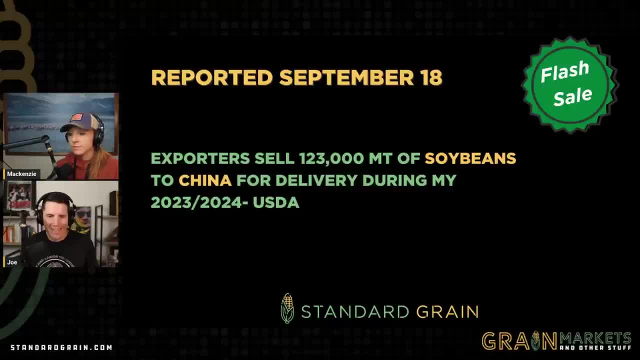 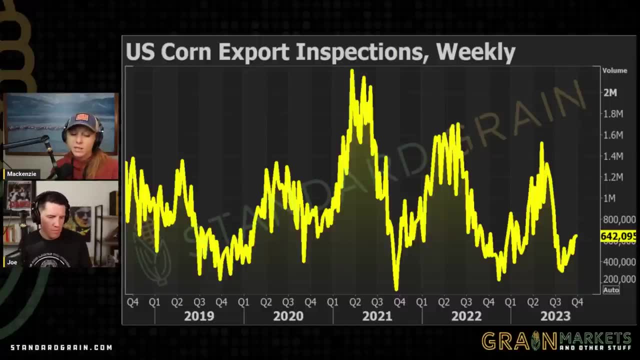 china or to somebody else, because our book of export sales is not where it needs to be at all. us corn shipments improved slightly last week. usda reported that 642 095 metric tons of corn were inspected for export during the week ending september 14th. the print was up 2.7.